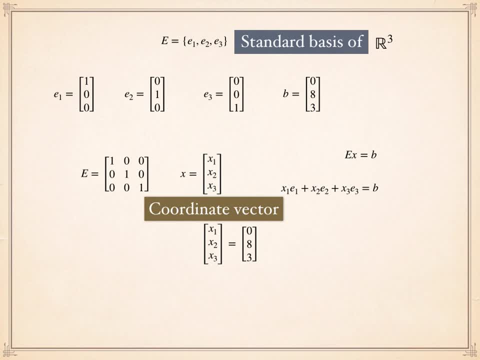 And the vector x actually is the same as vector b083.. Because if you want to do the calculation, if you take 0 times e1 plus 8 times e2 plus 3 times e3, you will get b. So the three values 0,, 8, 3 are the coordinates of vector b. 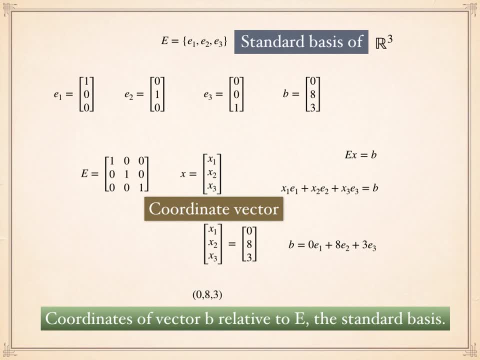 which is the standard basis of R3.. So keep in mind that if you're finding the coordinate vector for a vector in R3,, for an example, using the standard basis, the coordinate vector is the same as the vector that we're looking at. 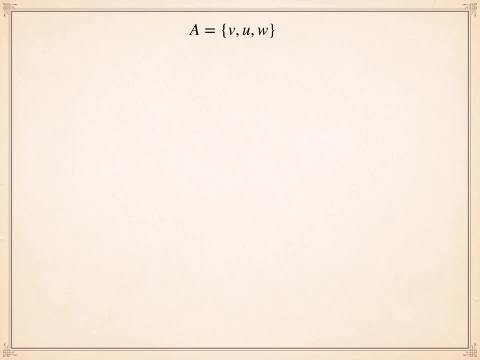 Now let's look at a different set of vectors: v, u and w. The first set of vectors is the set of vectors v, u, w, And also we're still looking at the same vector, b 0, h 3.. 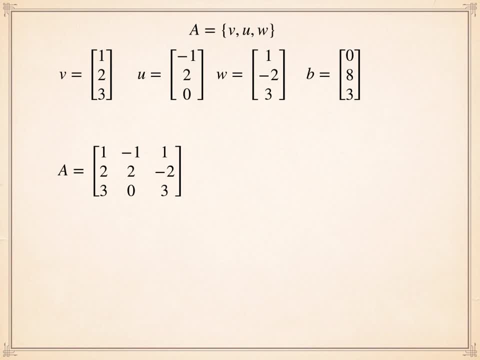 So from the three vectors v? u w, I can form a matrix A whose column vectors are v u w And I found the inverse matrix of A. So since I could find the inverse matrix of A, I know that this matrix is non-singular. 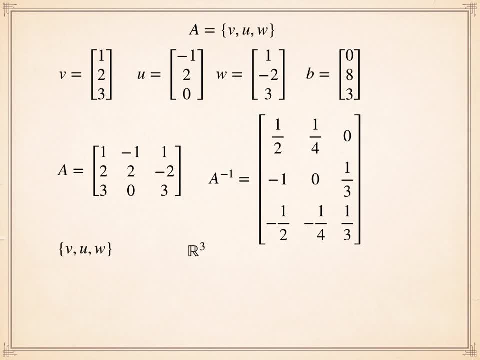 And since we're in R3 and we have three vectors, then the set of vector v u, w is a basis of R3. So we have another basis of R3. Now the question is: can we find a vector A such? 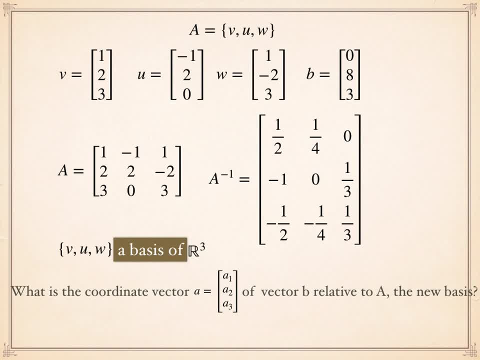 that A is a coordinate vector of b relative to A, the new basis, Or We find Scalars A1, A2, and A3 such that vector b is a linear combination of v, u and w vectors with weights of A1, A2, and A3, respectively. 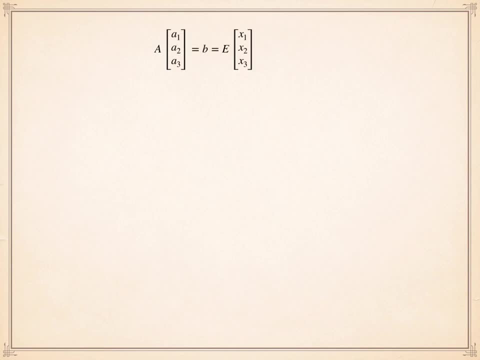 Well, let's look at an equation. We know that the matrix A multiplied to the vector A is equal to b, And also we already know that the matrix E, which is the identity matrix, that is formed by E1,, E2, and E3,. 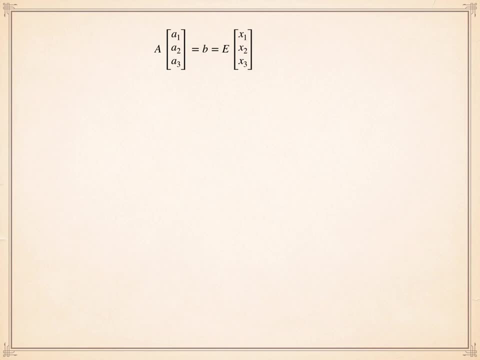 multiplied to the vector x, which is the coordinate vectors of b with respect to the standard basis, We found A inverse. We just multiply A inverse to this equation to solve for the vector A. It's clearly that vector A equals to A inverse times E times the x vector. 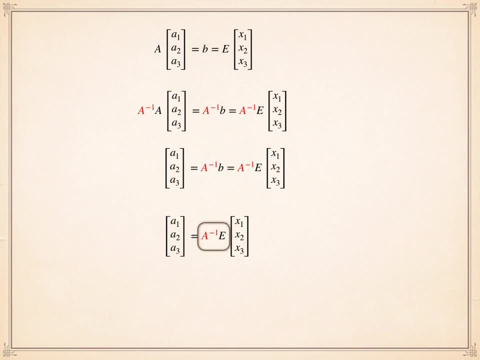 And if I set this matrix here A inverse times E, what I call it is an S matrix, And this matrix- S equals to A inverse times E- is actually the transition matrix from E to A, where E is the standard basis and A is a new basis. 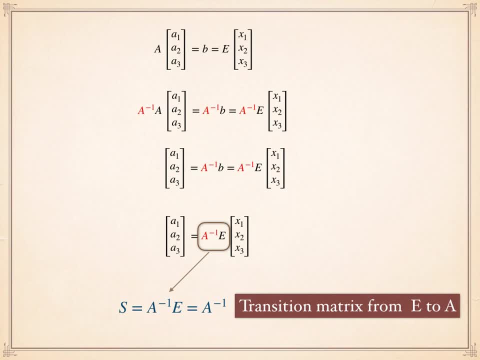 Because if you take this matrix, multiply to the coordinates with respect to E, you will get the coordinates with respect to A. So we call: S is the transition matrix from E to A. In order to find the vector A, I just need to use the inverse matrix of A and multiply to. 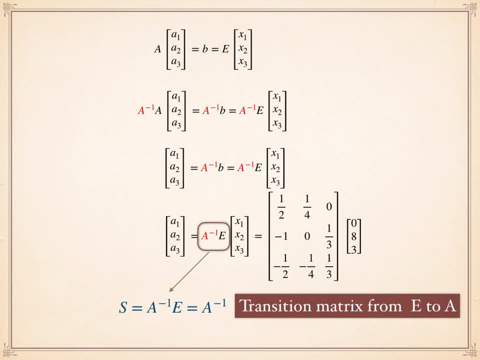 the x vector, which is the coordinate vector of vector b with respect to the standard basis, And this is 2, 1, negative 1, is the coordinate vector of vector b, And this is 2, 1, negative 1, is the coordinate vector of vector b. 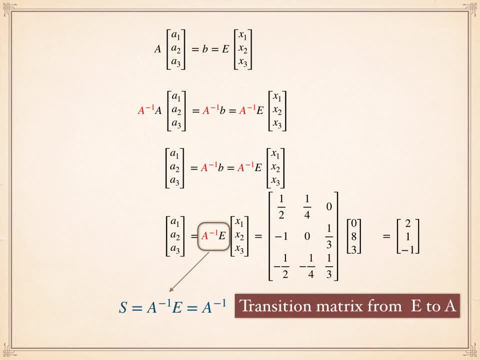 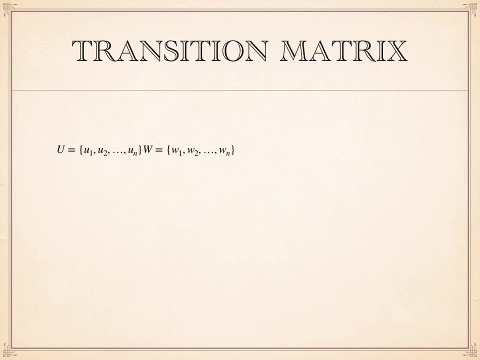 And this is 2,. 1, negative. 1, is the coordinate vector of vector b. With respect to the new basis, A is formed by u, v and w. So to summarize the idea of changing from one basis to another basis, 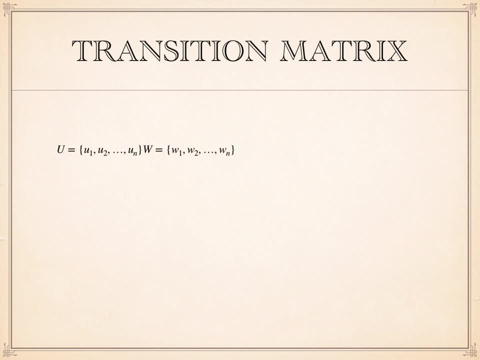 the idea of finding the new coordinates of a vector. with respect to the new basis, we can find the transition matrix. in general, If you have a two set of basis of a vector space, Then S equals to the inverse of w matrix times. the matrix u is the transition matrix. that helps translate the coordinates. 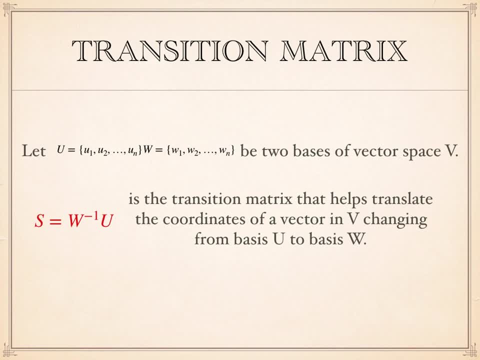 of a vector in the vector space v. changing from the basis u to basis w You the basis is very Gamut-AIDS. If you are representing your vector data from theUs andalf at inv to theV, you need to give dx. 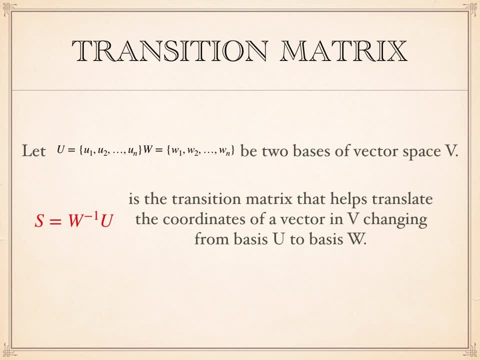 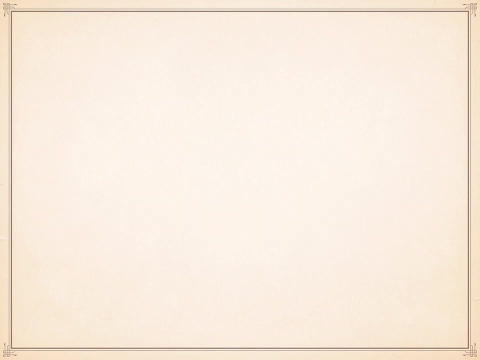 And u tolarausm should be equal to at U using the standard basis U, and if you want to change your basis from U to W, then you can use the transition matrix S equals to W inverse multiplied by U in order to translate all the coordinates from U to W. Well, let's look at an 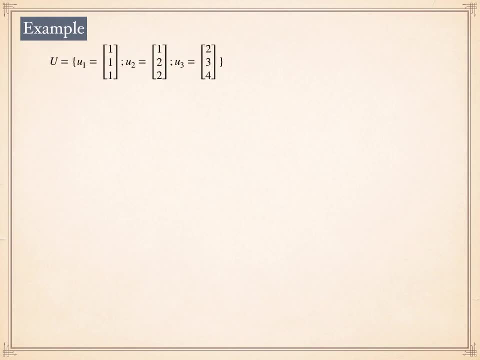 example. So I have a set of three vectors in U1 and W1,, W2 and W3.. I know that these two sets form basis of, So then my question is: can I find the transition matrix from U to W, And once I 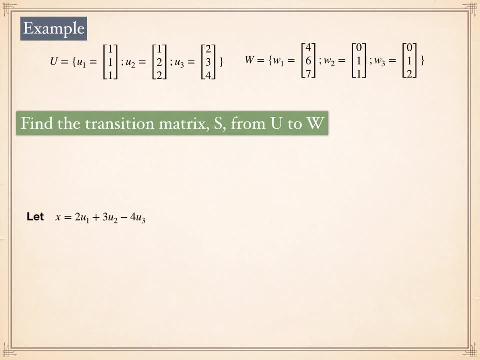 found the transition matrix. if I look at a vector x, it's a linear combinations of U1, U2 and U3, 3, with weights of 2,, 3, negative 1,. can I find the coordinates of x with respect to the basis w? 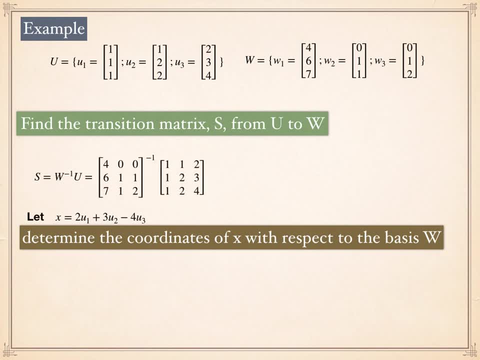 Well, let's find the transition matrix. So, by the definitions right, the transition matrix s equals to the inverse of w and multiplied to the matrix u, And we found that this is the transition matrix. And once we have the transition matrix, we can take the transition matrix multiplied by. 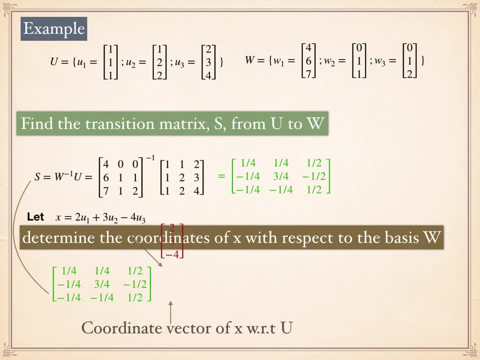 the coordinate vector of x with respect to u, which is 2,, 3, and negative 4, to find the coordinates of x, but with respect to the basis w, Again, in order to determine the new coordinates with respect to the new basis. 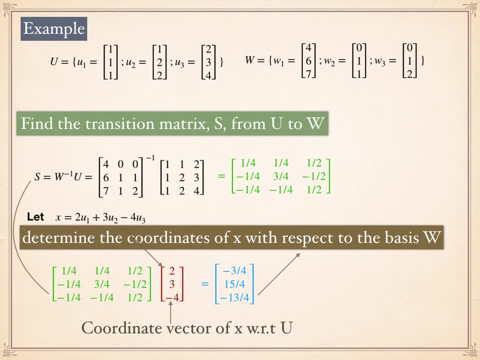 you find the transition matrix and then you multiply the transition matrix by the coordinates of the old basis to get the coordinates of the new basis. Here we go. you have it: the change of basis and how to find the transition matrix in a vector space. This is where we can consider what we can do to simplify the transition matrix.